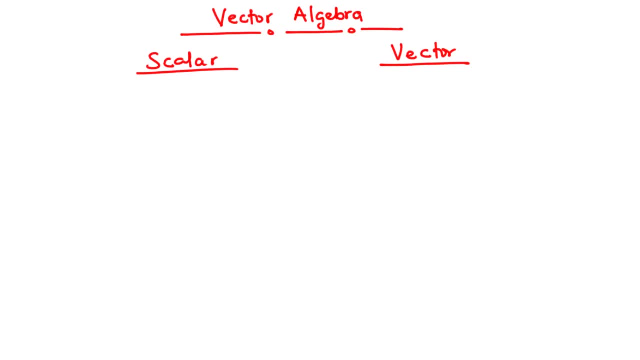 Now, if you are new here, make sure you subscribe to this channel, like this video and share this video to all your friends. Now let's get into today's lesson. What is the difference between a scalar quantity and a vector quantity? Now, a scalar quantity is a quantity that is completely defined by a single value. 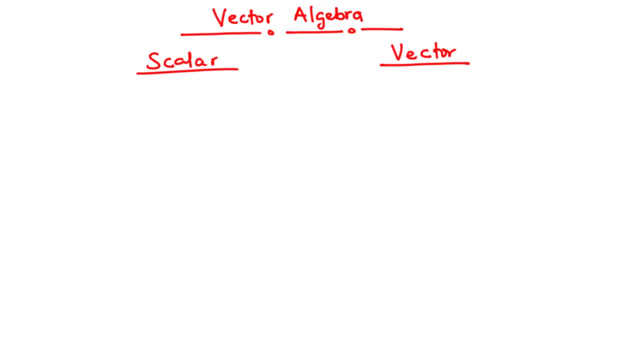 with an appropriate unit And we call this single value, the magnitude. Now examples of scalar quantities are: we have the length, mass, speed, and so on and so forth. Now we can talk about the length of a field to be 100 meters. 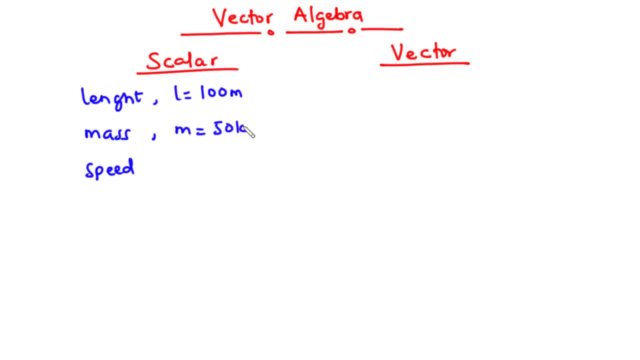 the mass of an object to be 50 kilograms, the speed of a car moving at 30 kilometers per hour. Now, these values, with their respective units, only specify the size or the magnitude of the quantities. Now, moving away from a scalar quantity, let's talk about 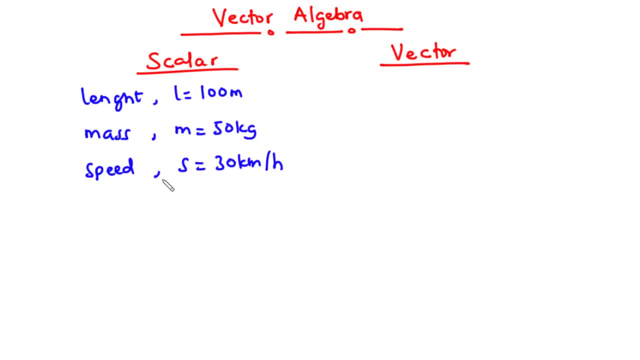 a vector quantity. Now, a vector quantity is a quantity that is completely defined when we know not only the magnitude but also the direction in which it operates. So examples of vector quantities are: we have velocity, that is speed in a specified direction. we have acceleration. 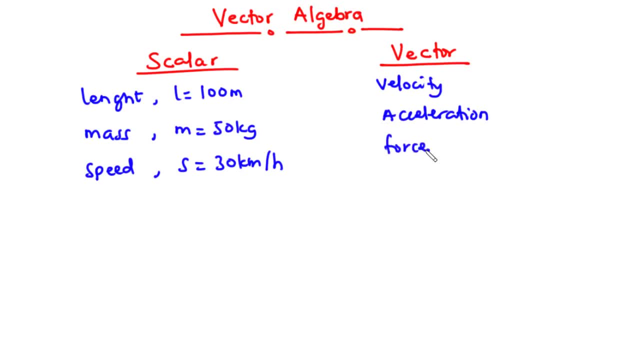 we have force and so on and so forth. So saying that the speed of a car is 30 kilometers per hour, this is a scalar and it only specifies the size or the magnitude of the quantity. However, we can talk of the velocity of a car to be 30 kilometers per hour, moving due east. 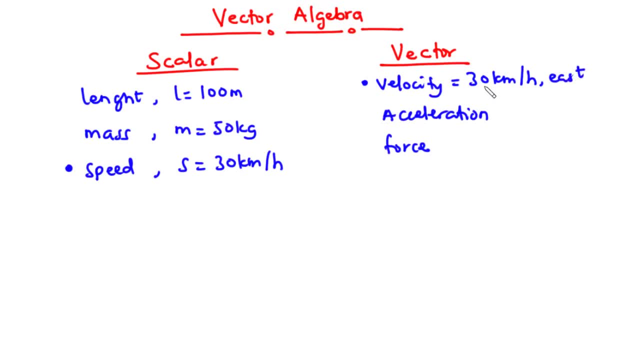 So this time we have a vector quantity which specifies both the magnitude and the direction which is due east. So, in summary, a scalar is a quantity which only specifies the size or the magnitude of the quantity, whereas a vector is a quantity which specifies not only the magnitude. 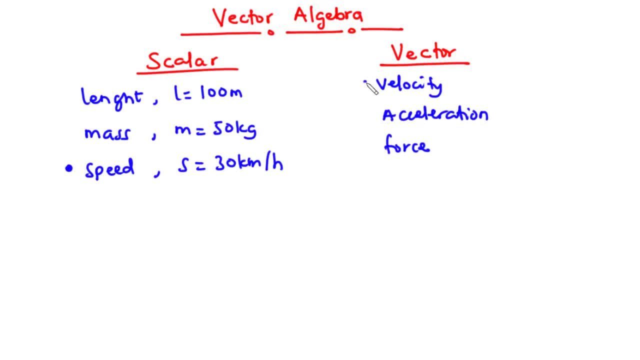 magnitude of the quantity. However, we can talk of the velocity of a car to be 30 kilometers per hour moving due east. So this time we have a vector quantity which specifies both the magnitude and the direction. So, in summary, a scalar is a quantity which only specifies the size or the magnitude of 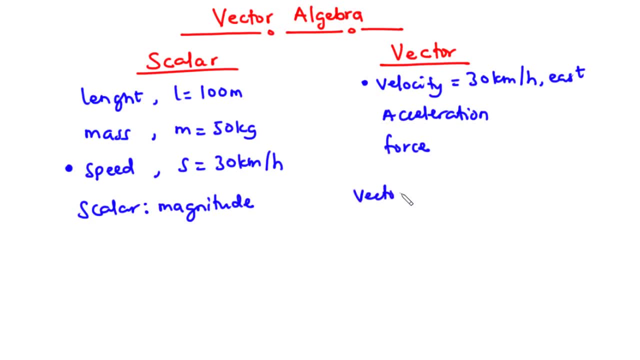 the quantity, whereas a vector is a quantity which specifies not only the magnitude but also the direction in which it operates. Now let's move on as we discuss some basic concepts of vectors. So let L be a straight line in a two or three dimensional space. 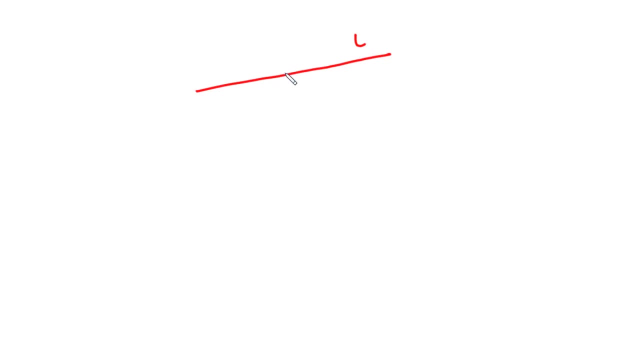 Now this line can have at most two directions, That is, it can either be directed this way or that way. Now this line with any of the two directions is called a directed line. Now let's assume that we have two points, Say A and B, on this line. 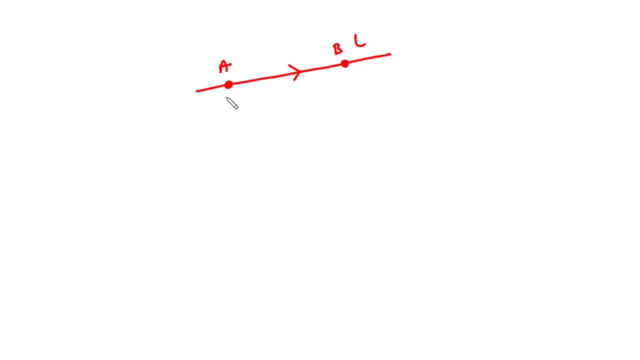 Then we are going to restrict the line L to the line segment AB so that we obtain a directed line segment. Now this directed line segment is called a vector in the sense that it has a magnitude, that is, the distance between the two points A and B. 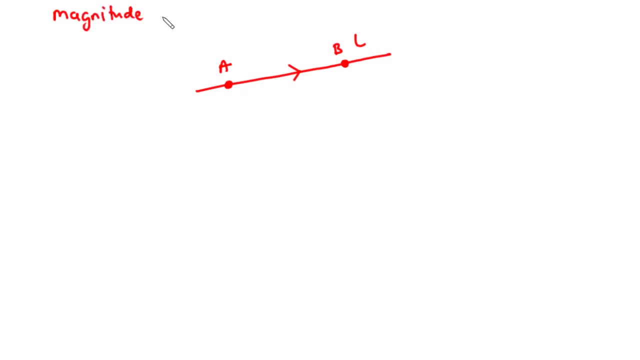 So that is called the magnitude And it also has a direction. Now this vector V is denoted as Vector AB and can be simplified as Vector A. So we call this Vector AB or simply Vector A, And the arrow basically indicates the direction of. 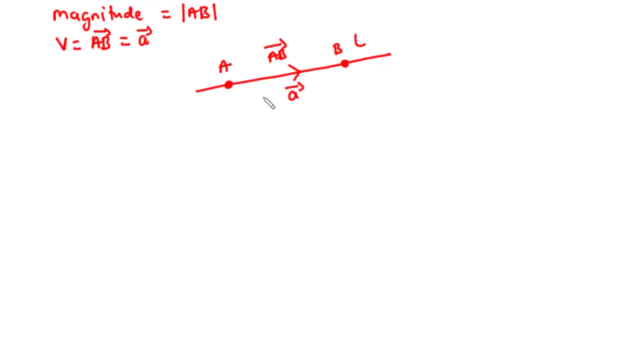 the vector. So the point from where the vector AB starts is called the initial point. The initial point starts when the vector A is in the direction of the vector, So this vector is directly denoted by the direction of the vector. and the point at B, where the vector ends, is called the terminal point. 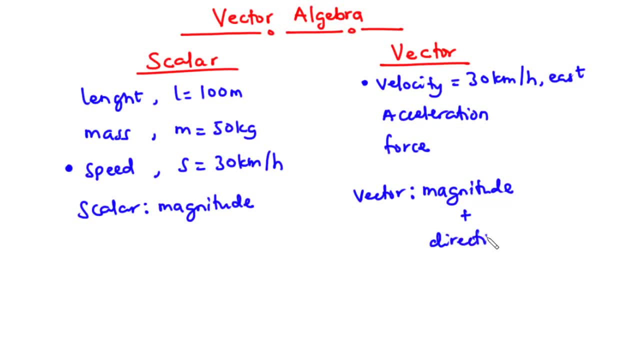 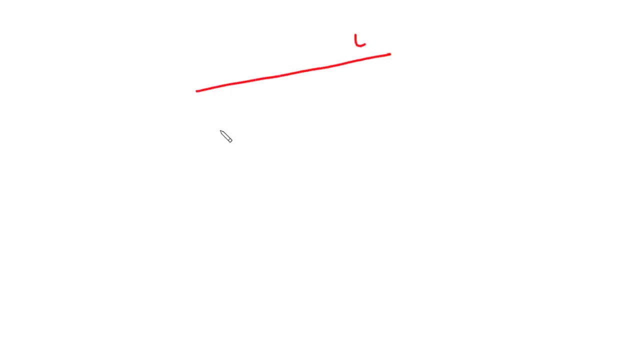 but also the direction in which it operates. Now let's move on as we discuss some basic concepts of vectors. So let L be a straight line in a two or three dimensional space. Now this line can have at most two directions, that is, it can either be directed this way or that way. 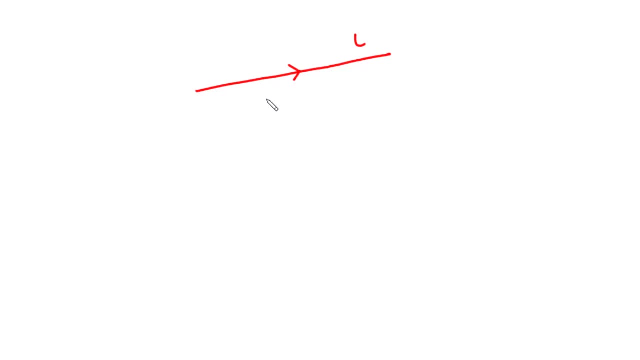 Now this line with any of the two directions is called a directed line. Now let's assume that we have a vector line here. two points, say A and B, on this line. Then we are going to restrict the line L to the line segment AB so that we obtain a directed line segment. Now this directed line segment is called a vector. 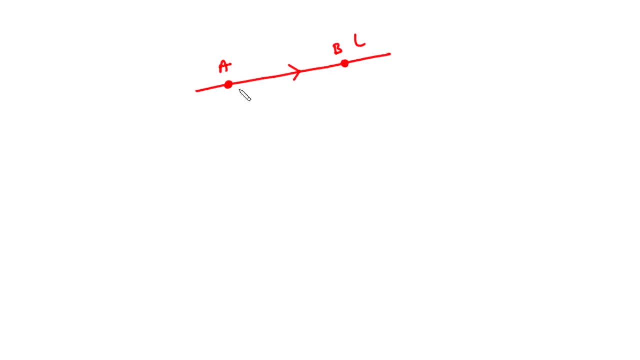 in the sense that it has a magnitude, that is, the distance between the two points A and B. So that is called the magnitude and it also has a direction. Now this vector V is denoted as vector AB and can be simplified as vector A. So we call this vector AB or simply vector A, and the arrow basically indicates the 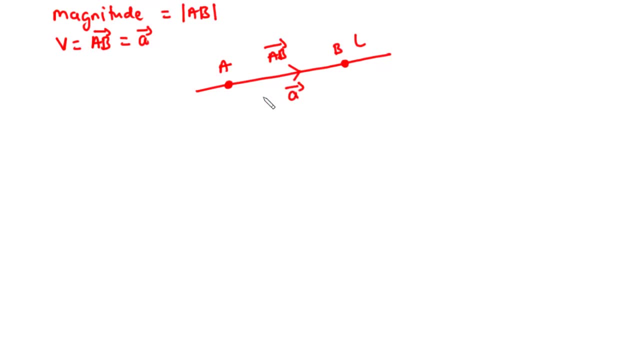 direction of the line segment. So we are going to restrict the line segment. So the point from where the vector AB starts is called the initial point and the point at B, where the vector ends, is called the terminal point. So we can represent the magnitude of the vector AB this way or, better still, we can simplify that as: 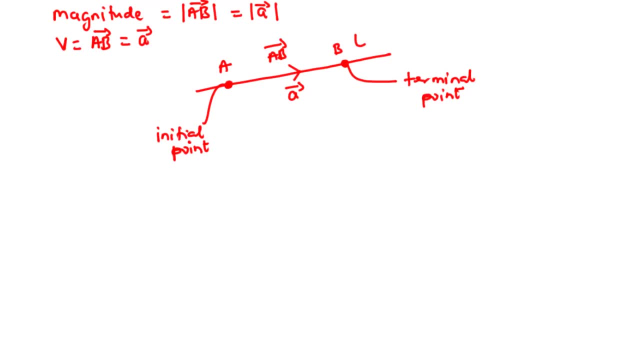 this. So how then do we find the magnitude of a vector? So, given two points, given two points, A and B, let's assume that we have A to be 2, 1, and then B to be 5, 4, and then we have vector V to be the directed line segment. 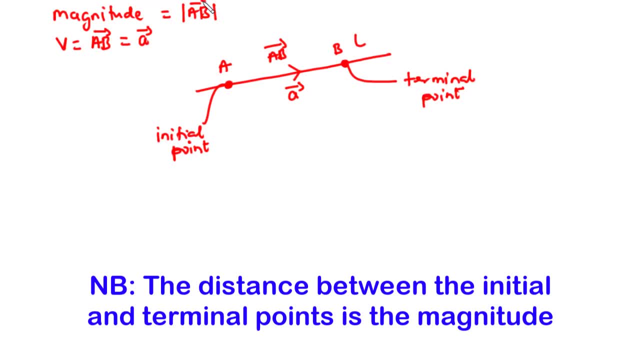 So we can represent the magnitude of the vector AB this way or, better still, we can simplify that as this: So how then do we find the magnitude of a vector? So, given two points, given two points, A and B, let's assume that we have A to be and 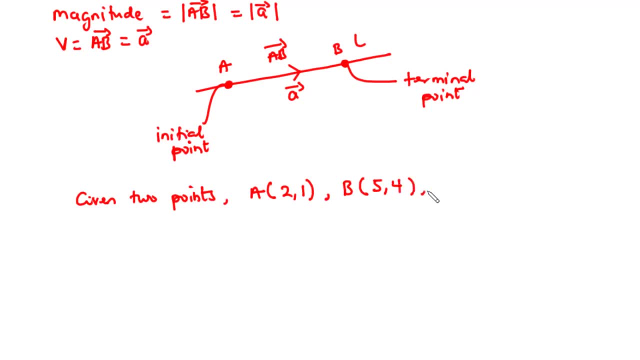 then B to be, and then we have vector V to be, the directed line segment from A to B. So now to find the magnitude of this vector, we first of all need to find the magnitude, to find the vector itself. Now, let's assume this to be the initial point and this to be the terminal point. 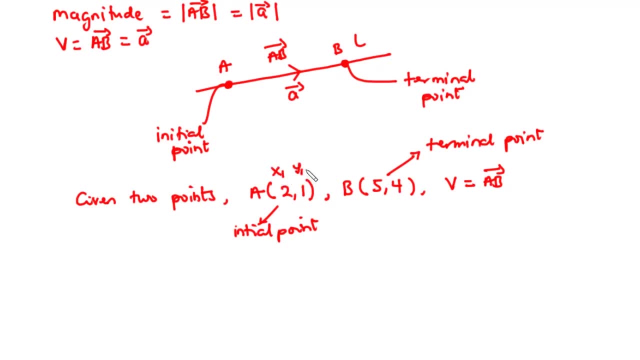 So in that sense, we have this to be X1, Y1 and then this to be X2, Y2.. Therefore, to find the vector that is given by vector V equals B. So what we do is we put the value of vector V to be the direct line segment from A to B. 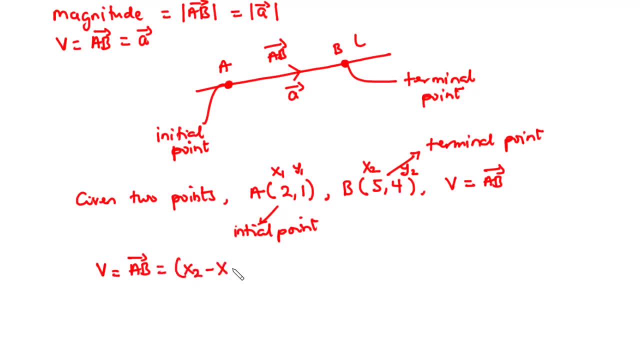 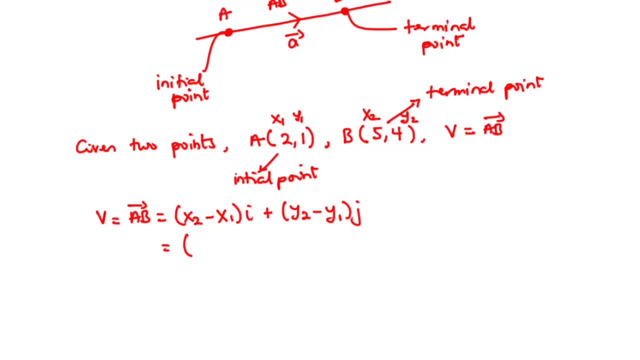 and that is equal to X2 minus X1 times I, plus Y2 minus Y1 times j. So let's substitute the values of X1, Y1, X2, Y2 in here. So that's going to be. we have X2 to be 5, X1 to be 2.. 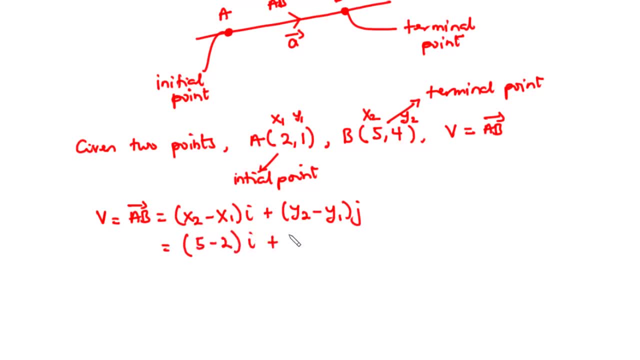 So that is 5 minus 2 times I. i plus we have y2 to be 4, y1 to be 1, so that is 4 minus 1 times j. so this becomes 3i plus 3j. so that is the vector ab and that is equal to vector v. now to find the magnitude of this vector. 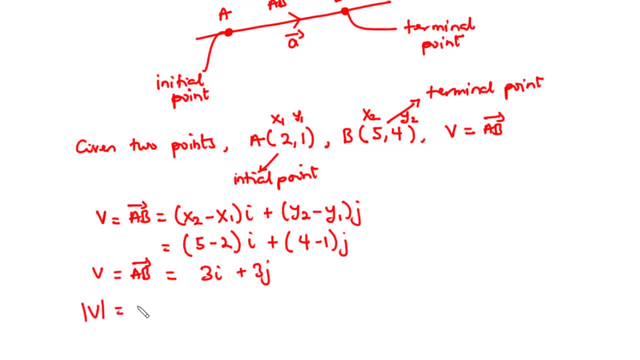 we say that the magnitude of vector v is equal to the magnitude of vector ab, and that is equal to the square root of the x component square plus the y component square. therefore, we have this to be the x component and this to be the y component. therefore, we have the magnitude of 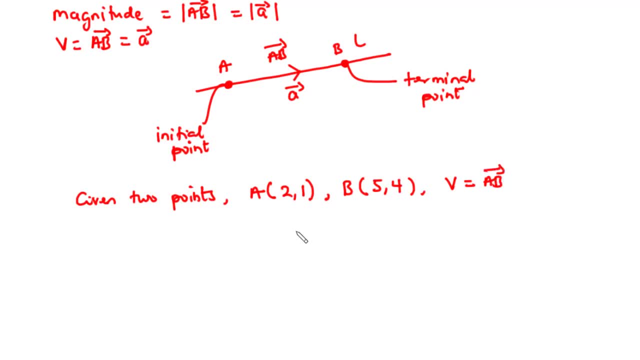 from A to B. So now to find the magnitude of this vector, we first of all need to find the vector itself. Now let's assume this to be the initial point and this to be the terminal point. So in that sense, we have this to be x1. 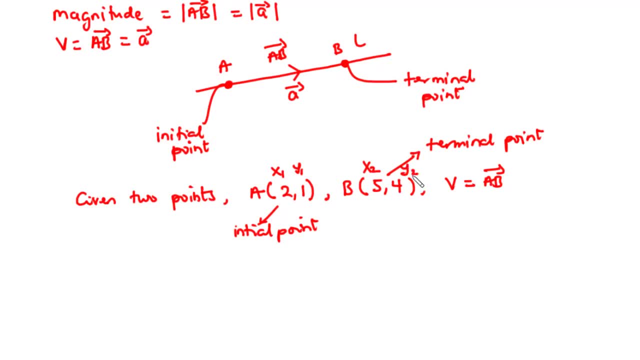 y1, and then this to be x2, y2.. Therefore, to find the vector that is given by vector V equals the directed line segment from A to B, and that is equal to x2 minus x1 times i, plus y2 minus y1 times j. So let's substitute the values of x1,y1, x2,y2. And then we have vector V stand in the direct line segment from A to B, which equals X2 minus X1 times i, Plus y2 minus y1 times j. So let's substitute the values of x1,y1, x2,y2,x0 and x. 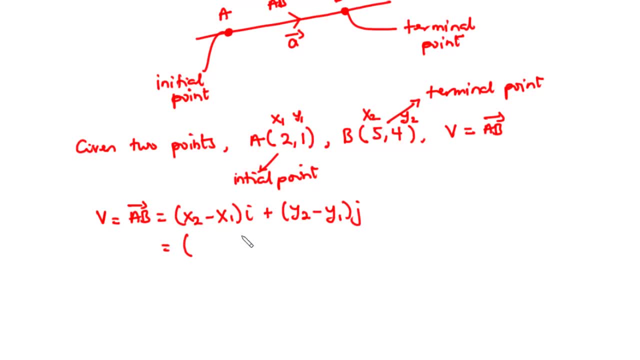 To find the erreicht line segment we need to find the initial point that was given by vector V, x2, y2 in here. so that's going to be. we have x2 to be 5, x1 to be 2, so that is 5 minus 2. 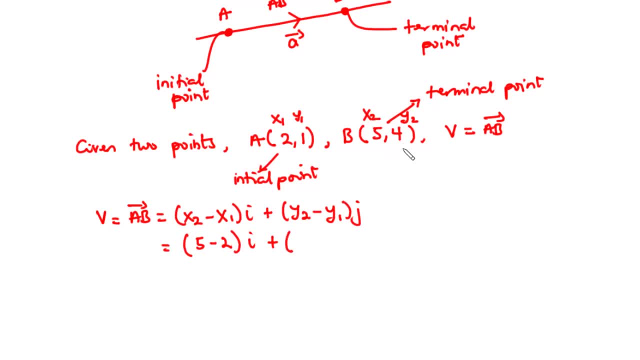 times i. plus we have y2 to be 4, y1 to be 1. so that is 4 minus 1 times j. so this becomes 3i plus 3j. so that is the vector ab and that is equal to vector vane. now to find the magnitude. 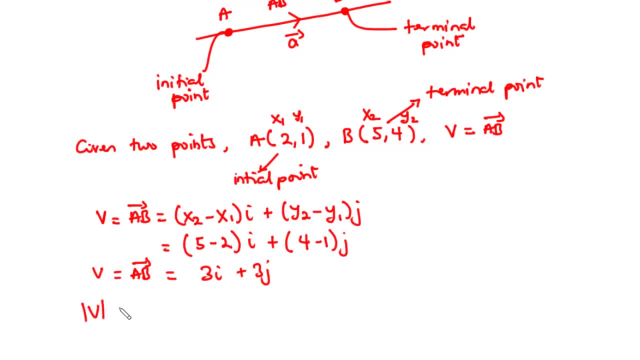 of this vector. we say that the magnitude of vector vane is equal to the magnitude of vector ab, and that is equal to the square root of the x component square plus the y component square. therefore, we have this two to be the x component and this to be the y component. therefore, we have the magnitude. 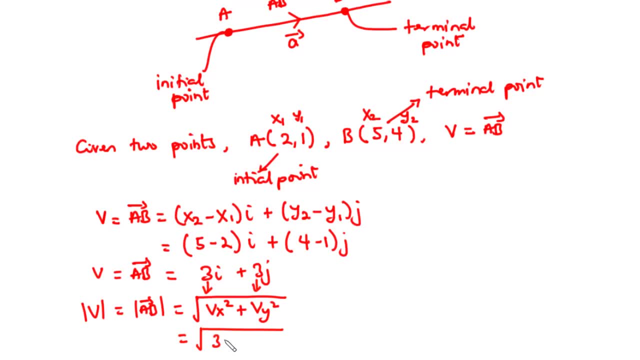 of vector vane to be equal to the square root of 3 square plus 3 square, and that is equal to 9 plus 9. now 9 plus 9 is equal to 18, and that can be simplified as 3 root 2. so we have: 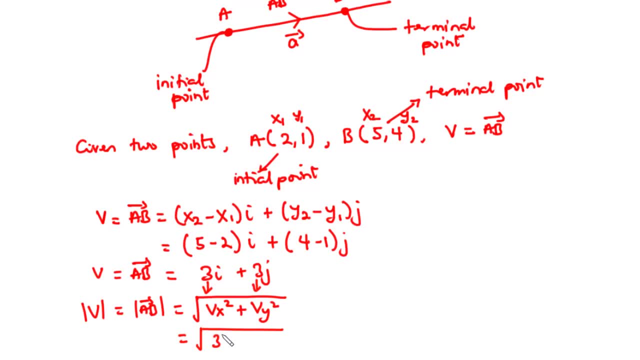 vector v to be equal to the square root of 3 square plus 3 square, and that is equal to 9 plus 9. now, 9 plus 9 is equal to 18, and that can be simplified as 3 root 2. so we have the magnitude of vector v, which is equal to the magnitude of vector ab, to be equal. 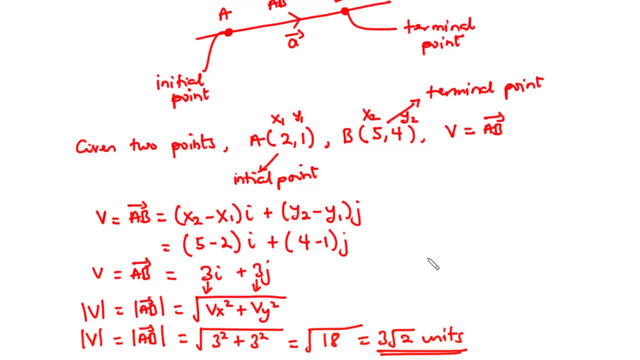 to 3 root 2 units. so in the same way, let's assume that we have a vector c, v with components v, two, three and six. therefore the vector v is equal to 2i plus 3j plus 6k. so how do we find? 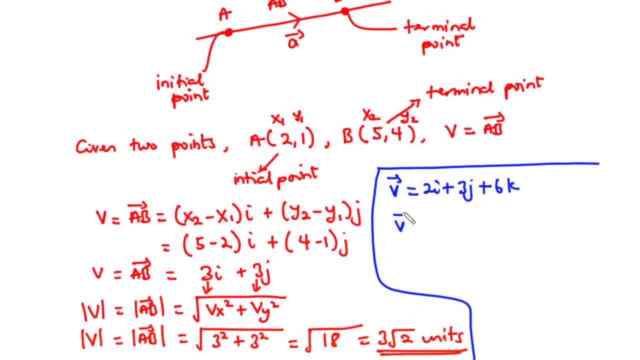 the magnitude of this vector. now, the magnitude of this vector is given by the square root of vx square plus vy square plus vz square. now let's substitute the values of vx, vy and then visit, so we are going to have the square root of 2 square plus 3 square plus 6 square, so that is equal to. 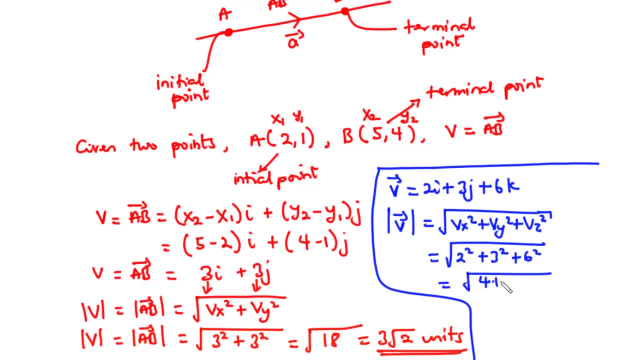 we have the square root of 2 square is 4, 3 square is 9, 6 square is 36.. now, 4 plus 9 is 13 plus 36 is 49. so that is equal to the square root of 49 and the square. 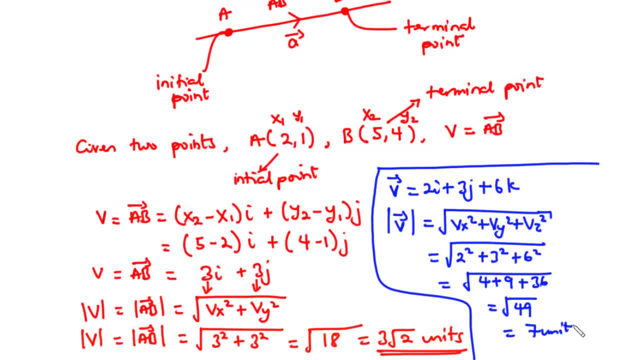 root of 49 is equal to 7.. so we have the magnitude of the vector v to be 7 units. now let's move on as we discuss the various types of vectors that are going to be useful to us in our subsequent lessons. now the first we are going to start off. 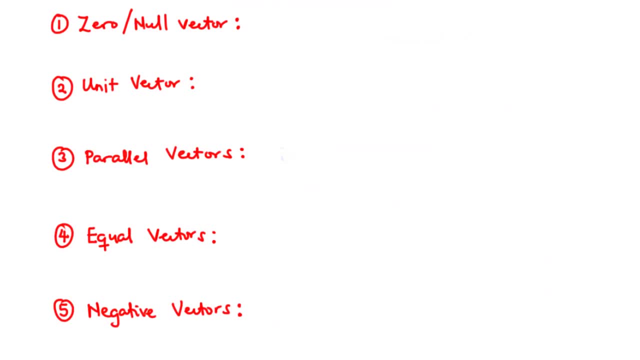 with is what we call the zero or the null vector. so the zero or the null vector is a type of vector whose initial and terminal point coincide. now this type of vector is denoted as zero with the arrow on top and is equal to 0: 0 in a two-dimensional space, or 0 0- 0 in a three-dimensional space. 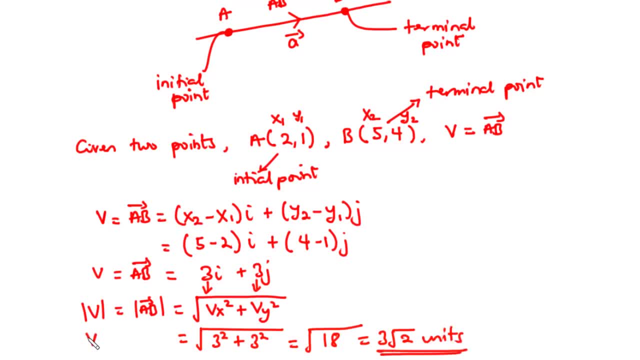 the magnitude of vector vane, which is equal to the magnitude of vector ab, to be equal to 3 root 2 units. so in the same way, let's assume that we have a vector saving with components 2, 3 and 6. therefore the vector vane is equal to. 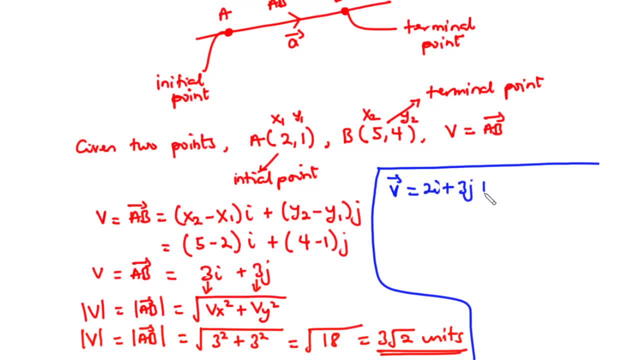 2i plus 3j plus 6k. so how do we find the magnitude of this vector? Now, the magnitude of this vector is given by the square root of vx square plus vy square plus vz square. Now let's substitute the values of vx, vy and then vz. 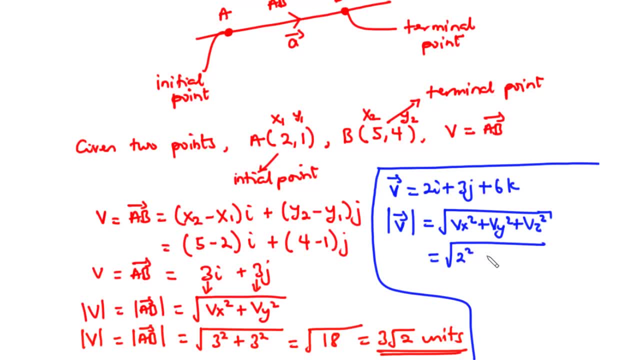 So we are going to have the square root of 2 square plus 3 square plus 6 square, So that is equal to. we have the square root of 2 square is 4,, 3 square is 9, 6 square is 36.. Now 4 plus 9 is 13. 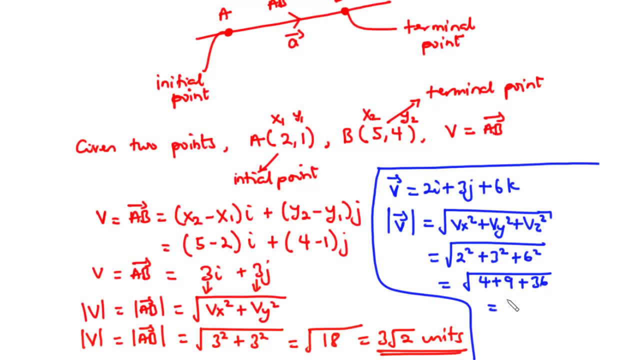 plus 36 is 49. So that is equal to the square root of 49, and the square root of 49 is equal to 7.. So we have the magnitude of the vector v to be 7 units. Now let's move on as we discuss. 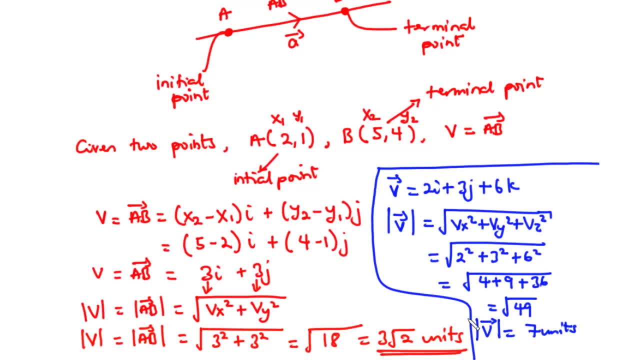 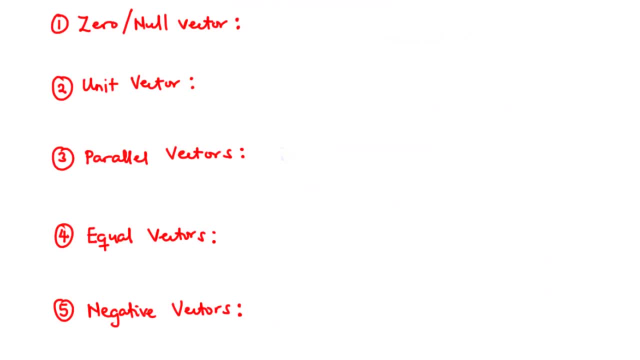 the various types of vectors that are going to be useful to us in our subsequent lessons. Now, the first we are going to start off with is what we call the zero or the null vector. So the zero or the null vector is a type of vector whose initial and terminal points coincide. 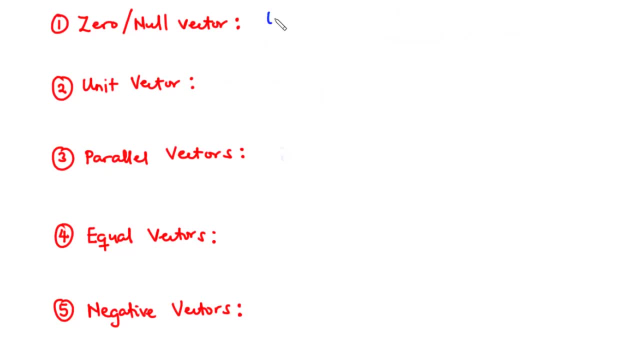 Now this type of vector is denoted as zero with the arrow on top and is equal to zero- zero in a two-dimensional space, Or zero, zero- zero in a three-dimensional space. Now, since this type of vector has zero components throughout, then it means that the magnitude of 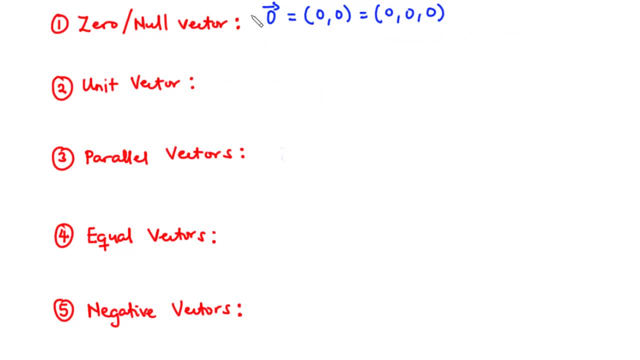 so this type of vector has zero components throughout, then it means that the magnitude of such a vector is equal to zero. so this vector has zero magnitude and has no specified direction. now let's move on to what we call the unit vector, whose magnitude is unity, or, better still, a vector whose magnitude is equal to 1.. 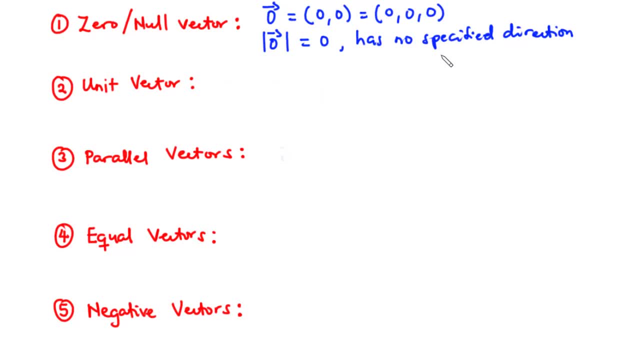 now, this unit vector is generally used to denote the direction of a vector, so that given a vector, say a, then the unit vector in the direction of this given vector is represented as a cap, and that is equal to the given vector divided by its magnitude. so this is the unit vector. 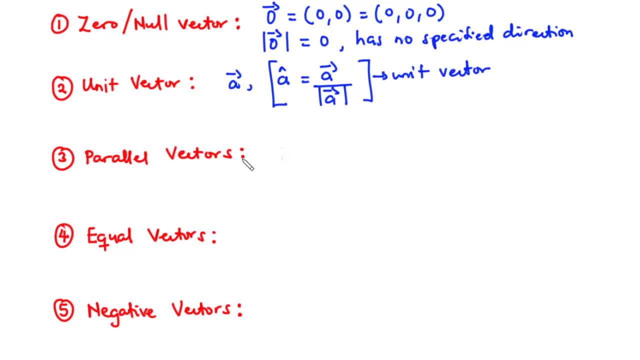 now let's move on to parallel vectors. now two vectors are said to be parallel if one is a scalar multiple of the other. so giving two vectors, say a and b, then we have vector a equals lambda times vector b, where lambda is the scalar or the number. 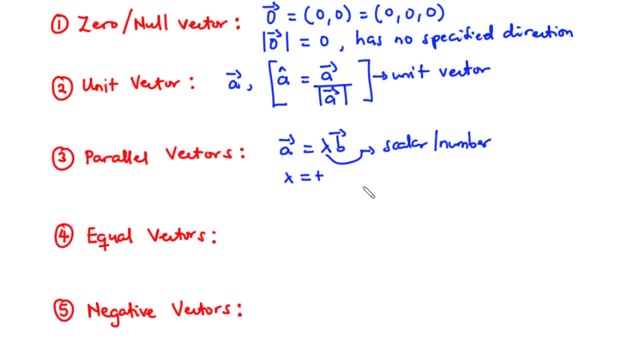 now, if lambda is positive, then what this primarily means is that the two vectors a and b are in the same direction. the two vectors a and b act in the same direction, but if the vector here is negative, then what this probably means is that the two vectors a and b 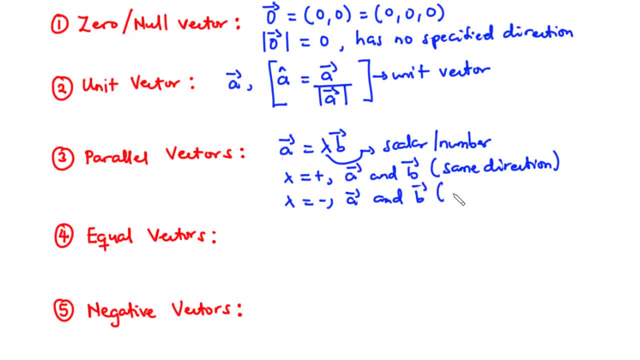 act opposite to each other. now to equal vectors. two vectors are said to be equal if they have the same magnitude, before and after, and direction. so given any two vectors, a and b, if these two vectors have the same magnitude and direction, then they are considered as equal vectors, which also means that 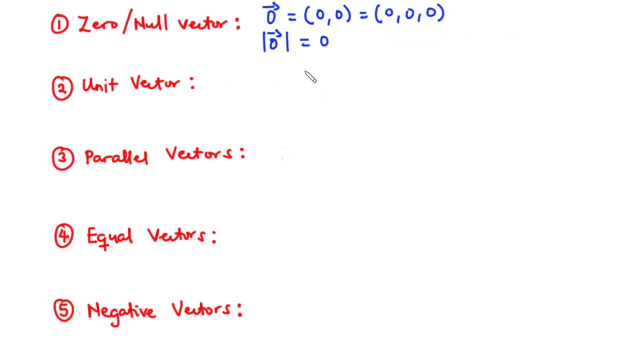 such a vector is equal to zero. So this vector has zero magnitude and has no specified direction. Now let's move on to what we call the unit vector. Now, a unit vector is a vector whose magnitude is unity or, better still, a vector whose magnitude is equal to one. Now, this unit vector is generally. 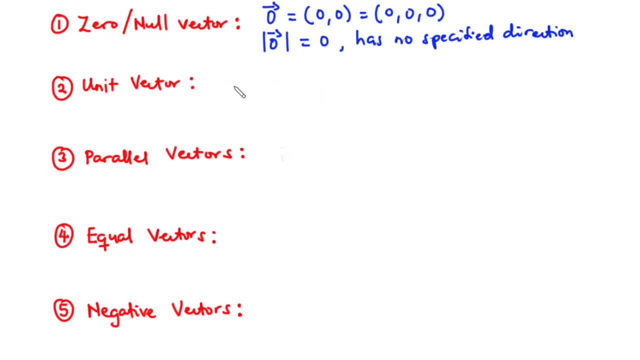 used to denote the direction of a vector, So that given a vector, say a, then the unit vector in the direction of this given vector is represented as a cap, and that is equal to the given vector divided by its magnitude. So this is the unit vector. 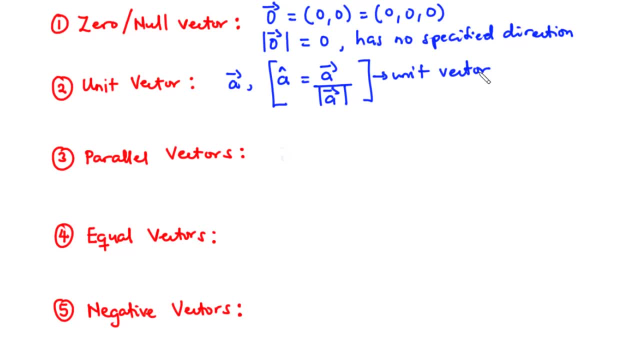 Now let's move on to parallel vectors. Now two vectors are said to be parallel if one is a scalar multiple of the other. So given two vectors, say a and b, then we have vector a equals lambda times vector b, where lambda is the scalar or the number. 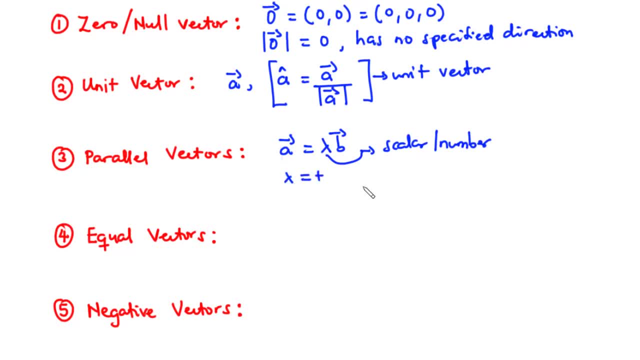 Now, if lambda is positive, then what this primarily means is that the two vectors a and b are in the same direction. The two vectors a and b act in the same direction. However, if lambda is negative, then what this probably means is that the two vectors a and b act opposite to each other. 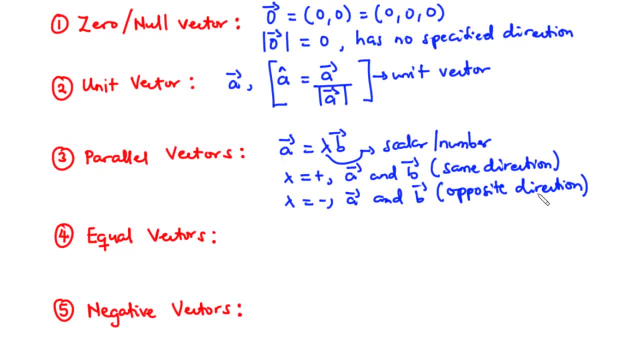 Now to equal vectors. So two vectors are said to be equal if they have the same magnitude and direction. So, given any two vectors, a and b, if these two vectors have the same magnitude and direction, then they are considered as equal vectors, Which also means that 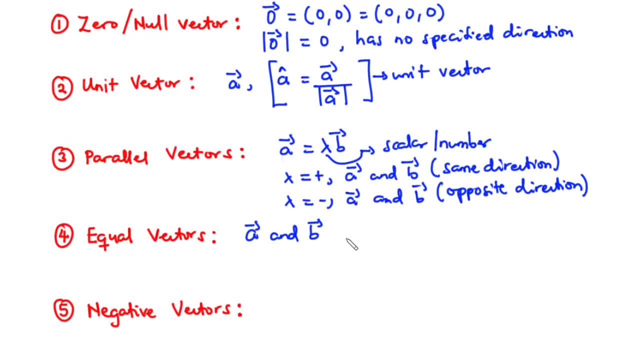 their corresponding components are also equal. So, given that vector a has components x1, y1, and 2, y1 and vector b has components x2, y2.. Now, if these two vectors are considered equal, then it means that x1 is equal to x2.